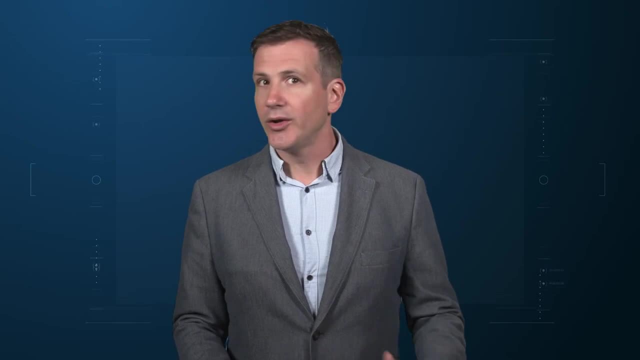 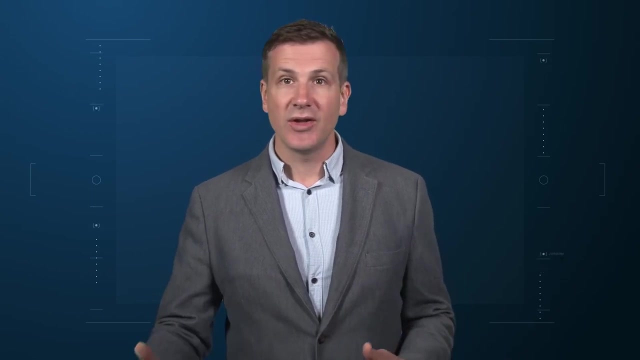 the cold hard arithmetic of transplant scarcity with the cold hard arithmetic of a computer algorithm ranking individuals on the wait list on a variety of factors, to ensure that those who will benefit most from a transplant get it first. But according to a new study, 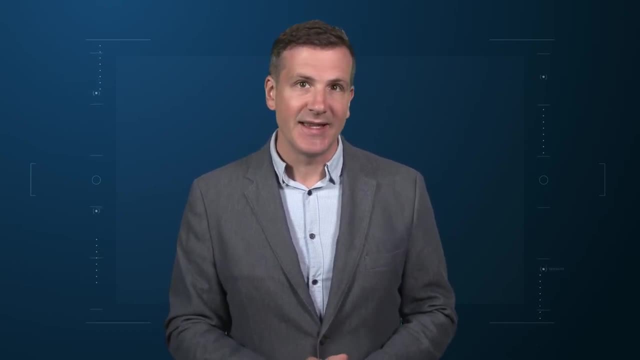 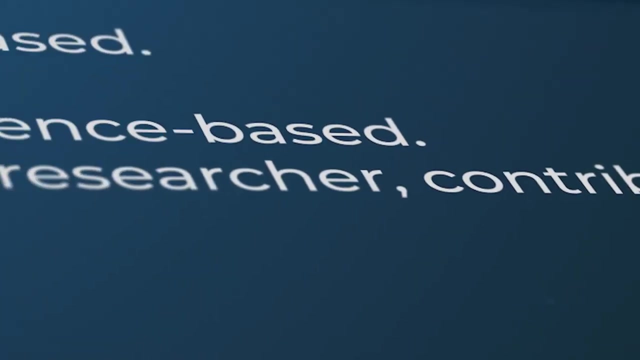 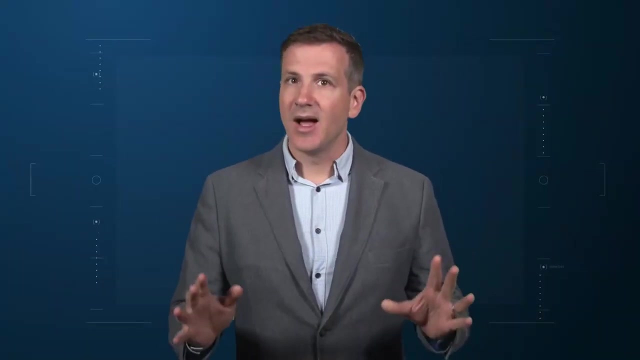 in JAMA Network Open. some centers seem to be treating this list as more of a suggestion than a rule, And that could be a real problem. This area is a bit complex, but I'll try to break it down into what you need to know. 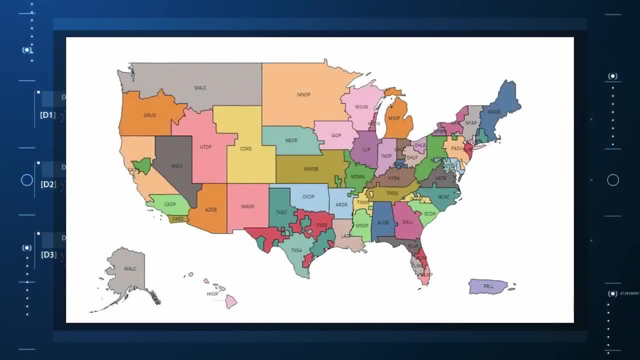 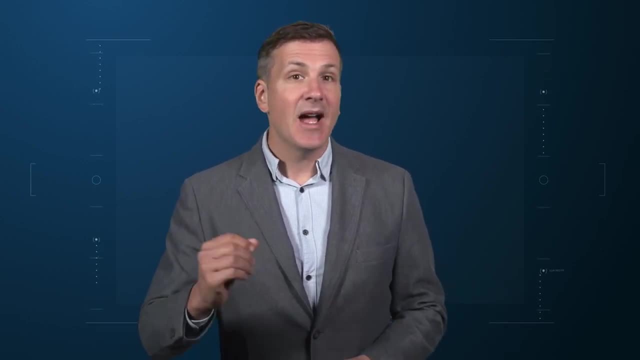 There are 56 organ procurement organizations in the US. These are non-profits with the responsibility to recover organs from deceased donors in their area. Each of those OPOs maintains a ranked list of those waiting for a kidney transplant. Depending on the OPO, the list may range from a couple of hundred people. to a couple of thousand, but one thing is the same, no matter what, If you are at the top of the list, you should be the next to get a transplant. Most OPOs have multiple transplant centers in them and each center is going to prioritize. 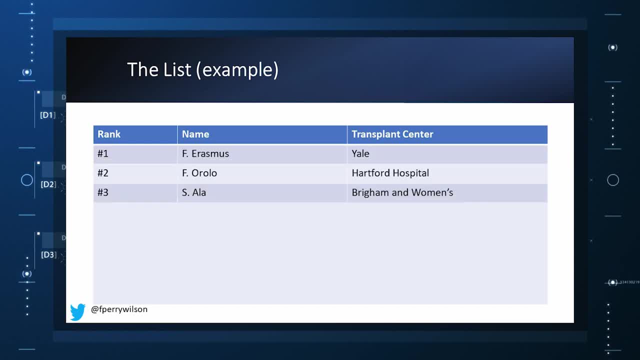 their own patients. If a Yale patient is number one on the list and a kidney offer comes in, it would be a good idea for us to accept, because if we reject the offer, the organ may go to a competing center whose patient is ranked number two. 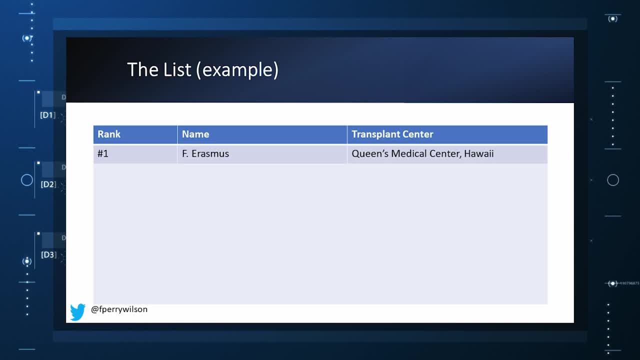 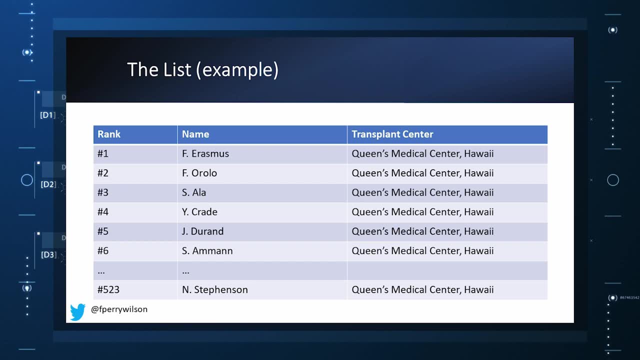 But 11 OPOs around the country are only served by one center. This gives that center huge flexibility to determine who gets what kidney, because if they refuse an offer for whoever is at the top of their list, they can still give the kidney to the second person on their 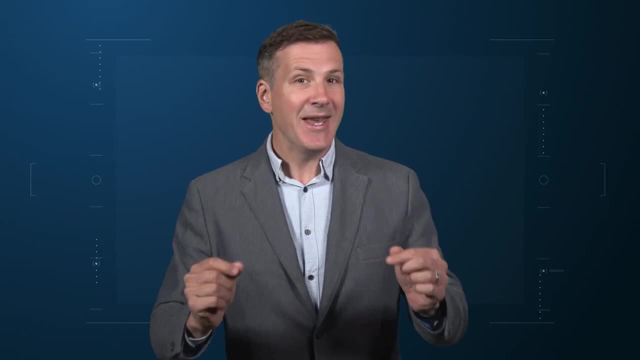 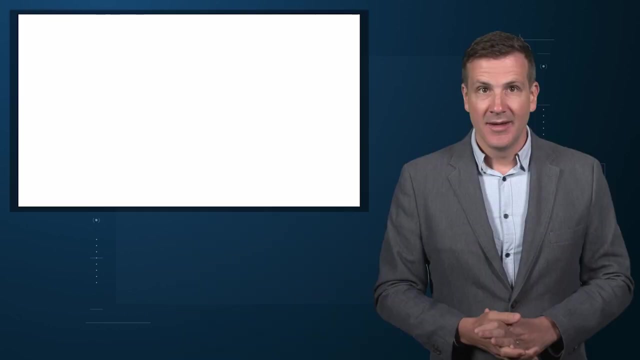 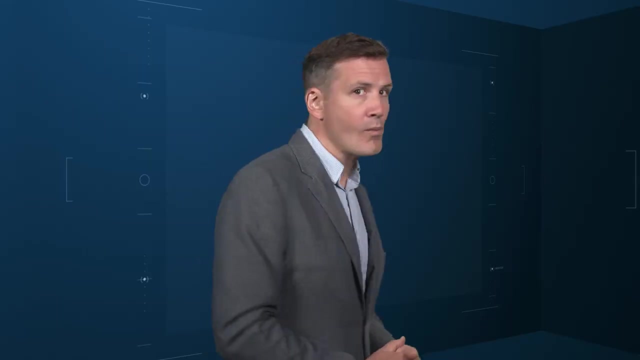 list or third or thirtieth, theoretically, But in practice, does this phenomenon, and often known colloquially as list diving, actually happen? This manuscript from Sumit Mohan and colleagues suggests it does, and at rates that are, frankly, eye-popping. The Columbia team used data from the Scientific Registry of Transplant Recipients to conduct the analysis. The database tracks all aspects of the transplant process, from listing to ranking to, eventually, the transplant itself. With that data, they could determine how often, across these 11 OPOs, did the transplant process go wrong. 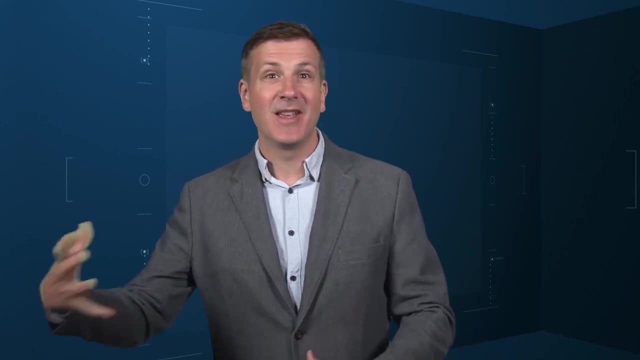 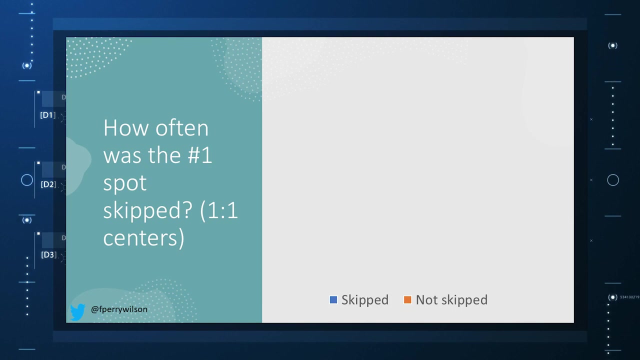 The data is also used to determine how often a patient was at the top of their list, and could the number one person on the list not get the available kidney? The answer Out of 4,668 transplants conducted from 2015 to 2019,. the transplant centers. 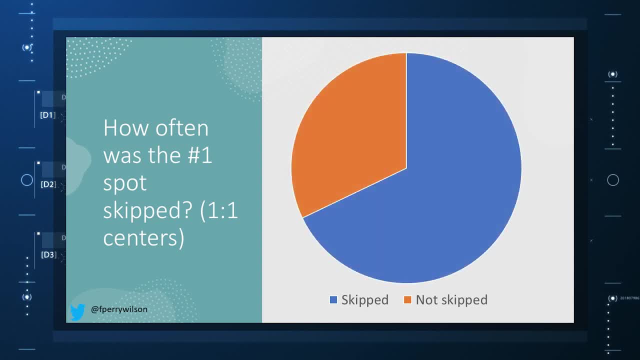 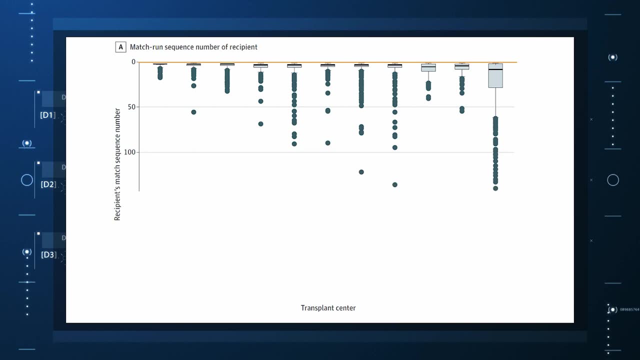 skipped their highest ranked person 3,169 times 68% of the time. This graph shows the distribution of where on the list these kidneys went. You can see some centers diving down 100, 200 places. Transplant centers have lists of differing lengths. 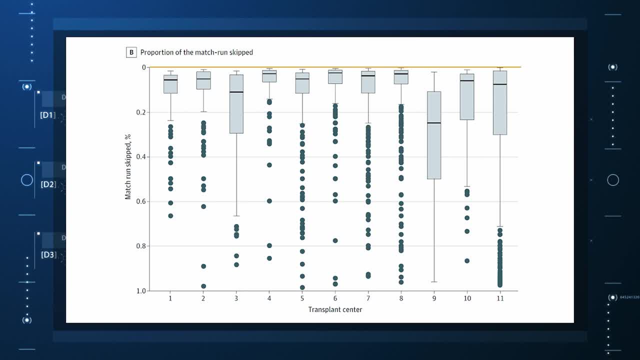 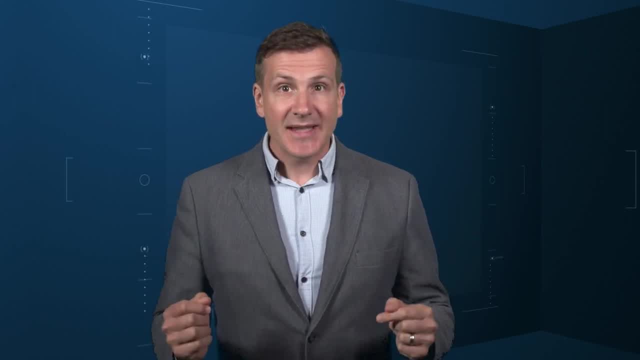 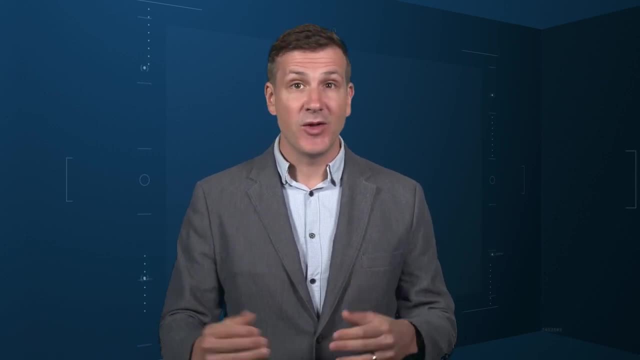 So this graph shows you how far down on the percentage scale the centers dived. You can see centers skipping right to the bottom of their list in some cases. Now I should make it clear that transplant centers do have legitimate discretion here. Transplant centers may pass up a less than perfect kidney for their number one spot. knowing that that individual will get more offers soon in favor of someone further down the list who will not see an offer for a while. It's gaming the system a bit, but not for evil, And the data supports this. Top-ranked people who got skipped had received a lower quality. 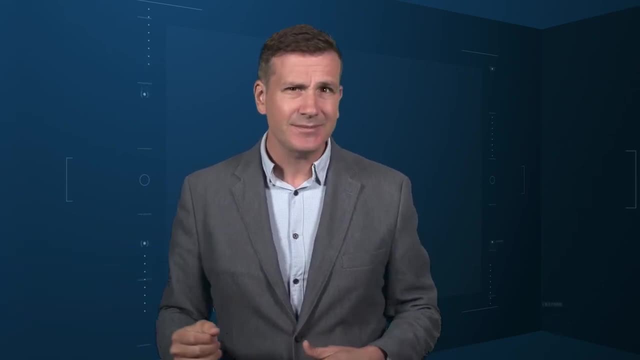 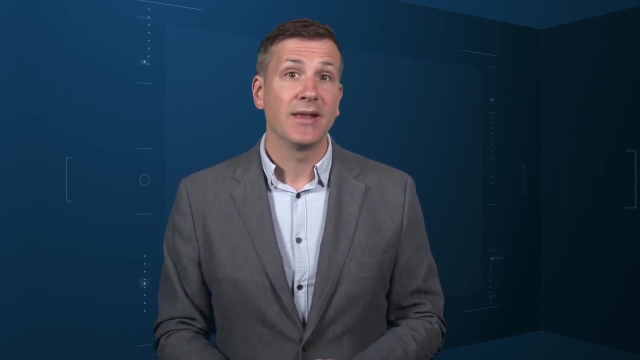 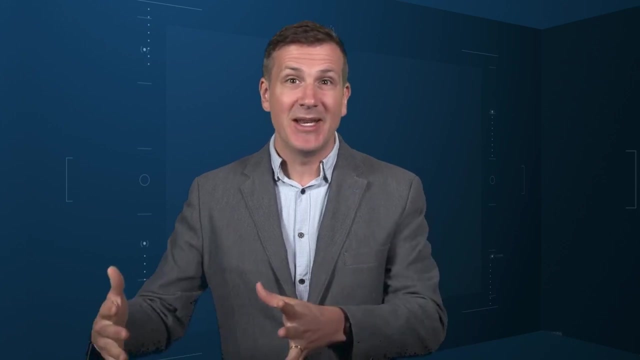 kidney offer than top-ranked people who did not get skipped. But I will also note that those who were skipped were less likely to be white, less likely to be Hispanic and more likely to be male. That should raise your eyebrows. Interestingly, this practice may not be limited to those cases where the OPO has only one. 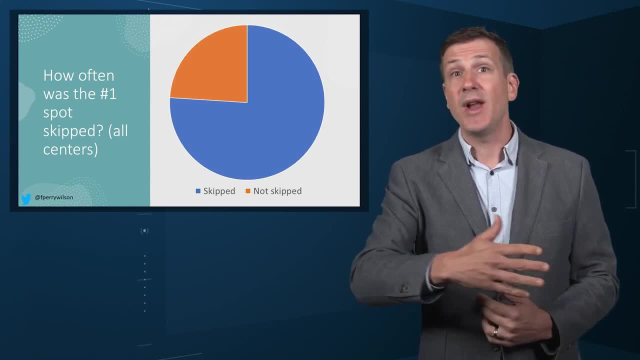 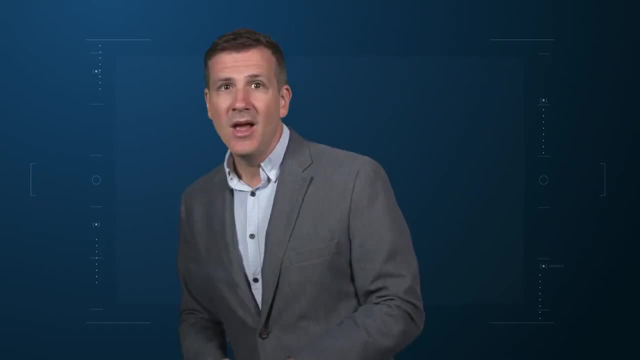 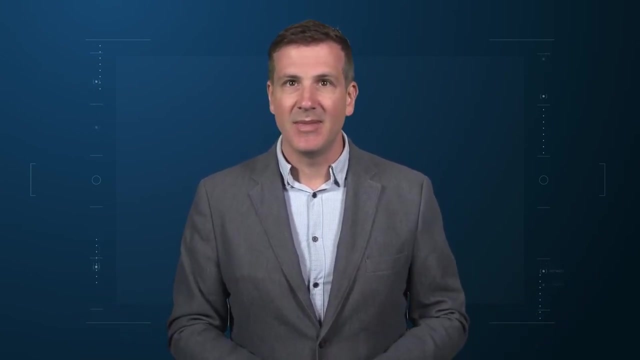 transplant center. Conducting the same analysis across all 231 kidney centers in the US, the authors found that the top candidate was skipped 76% of the time. So what's going on here? I'm sure that some of this list skipping is for legitimate medical reasons, and it should be pointed out that recipients have a right to refuse an offer as well and might be more picky if they know they are at the top of the list. But patient preference was only listed as the reason for list diving in about 14% of. 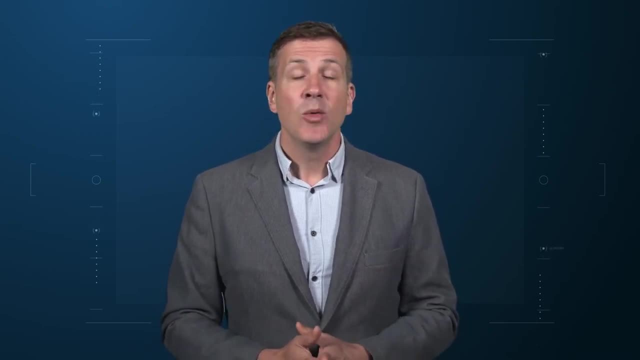 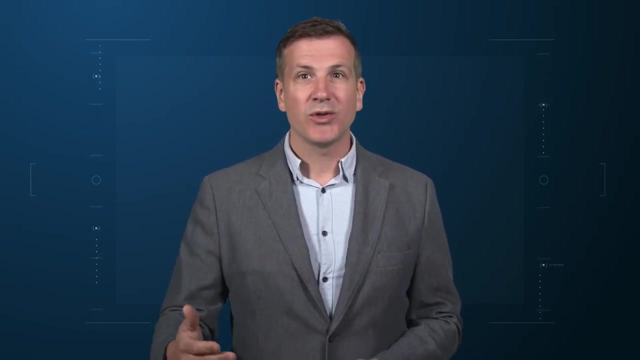 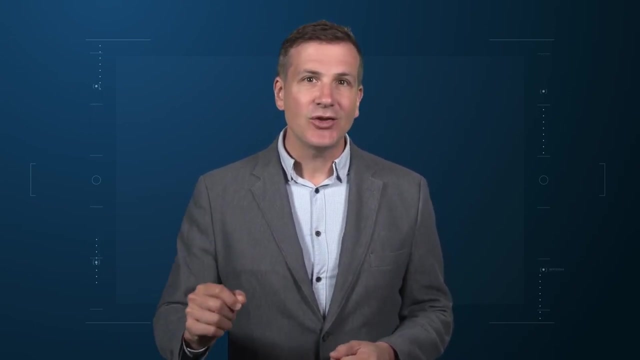 cases, For the vast majority of reasons listed, 65% were based on donor quality. The problem is that that can be quite subjective, And remember these organs were transplanted eventually, so they couldn't have been that bad. Putting the data together, though, I can't shake the sense that centers are using the 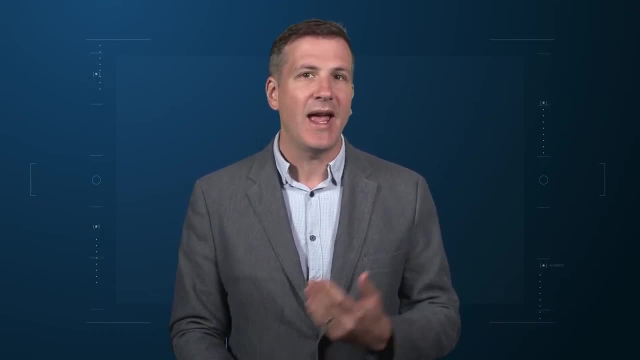 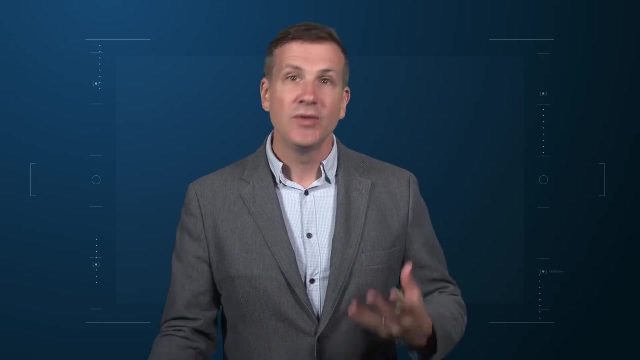 list more for guidance than as a real mechanism to ensure an equitable allocation system. With all the flexibility, centers have to bypass individual people on the list, the list loses its meaning and its power. I spoke to one transplant nephrologist who suggested this data should prompt an investigation. 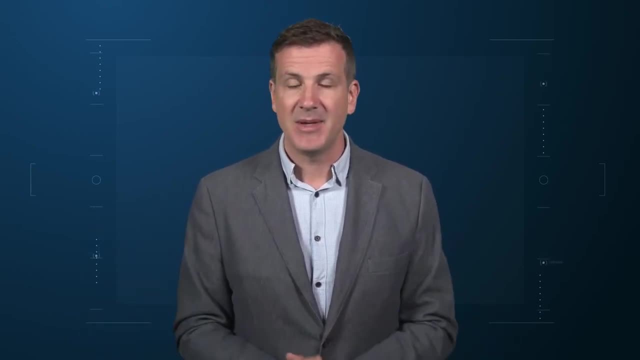 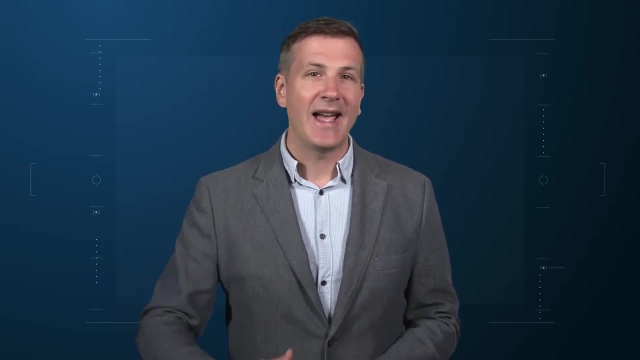 by UNOS, the body that governs all these OPOs. That may be a necessary step. Look, I hope there comes a day when this issue is moot, when growing kidneys in the lab or regenerating one's own kidneys is a possibility. 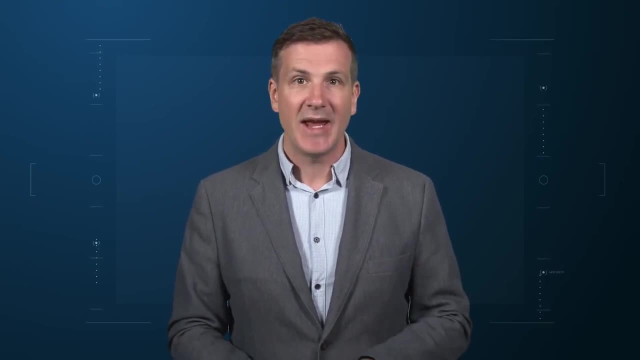 But that day is not yet here and we must deal with the scarcity we have In this world. we need the list to prevent abuse, But the list only works if the list is followed. The list only works if the list is followed.